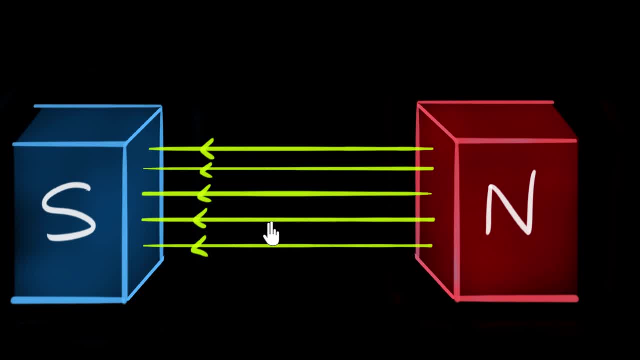 start curving like this, but at least in the center of the field will be straight. it will be easier to analyze what direction the current will be. and for the for to induce a current we need a coil. but instead of a coil we can just move a wire. so let's introduce a wire over here and we can move this. 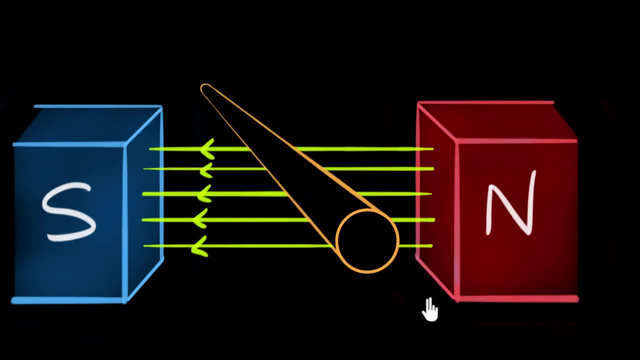 wire up and down like this. so as we move this wire notice it starts cutting the magnetic field and whenever it does that an electric current will be induced in this wire. of course we need a closed circuit for that, so we can imagine the wire from here gets. 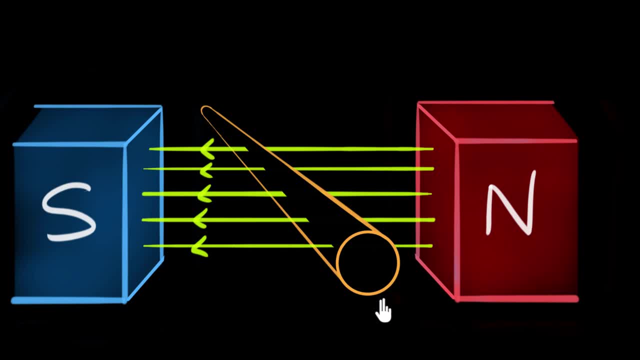 connected to some galvanometer somewhere which I've not shown over here. so let's say, we move this wire up like this: we move the wire up, so we push it up. then it turns out, if you do the experiment, the current generated in this wire, the current induced in this wire, is going to. 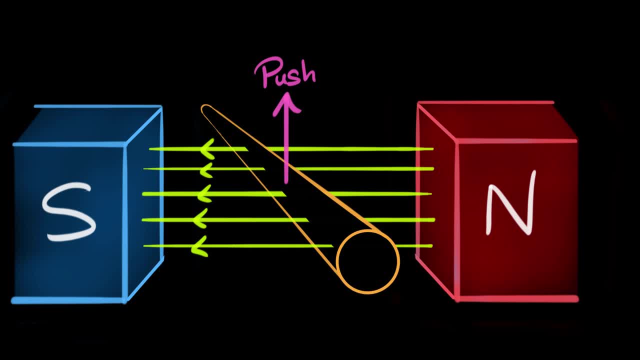 generate a current in this wire and the current induced in this wire is going to generate a current to be out of the screen. all right, somewhat like this. so the current will flow out of the screen this way and if you were to push it down, the current will reverse. the current direction will. 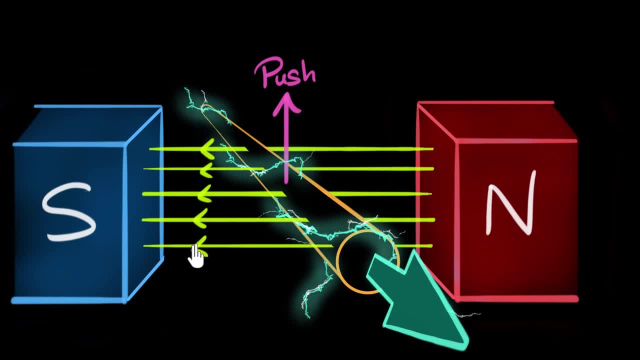 also depend upon the direction of the magnetic field. if you reverse the direction of the magnetic field, the whole current again will reverse. so now the big question is: how do we remember this? we will not worry about why the current is outwards, we'll just remember that the current is outwards. 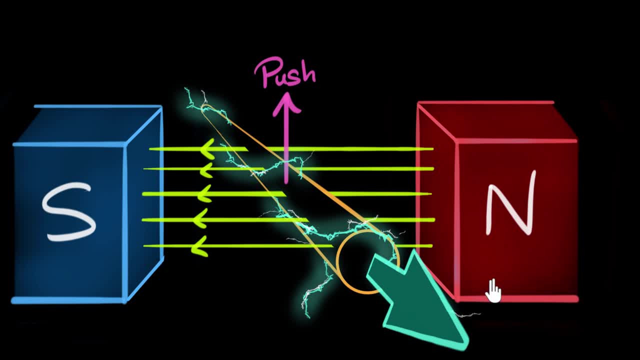 we'll just say that the experiment shows that it shows us it's that way. but how do you remember this? that's the big question we want to answer. so this can be remembered by using something called the right hand generator rule. so what we do is we take our right hand and we stretch the three. 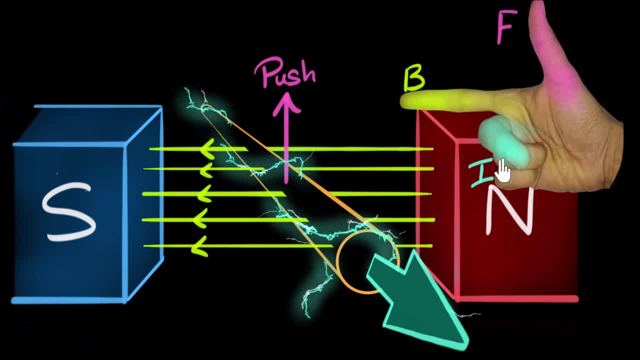 fingers- the thumb, the forefinger and the middle finger- this way such that they are perpendicular to each other, all of them. so this is perpendicular to this. this is perpendicular to this, if you see carefully. and even these two are perpendicular to each other. stress them that they're all perpendicular to each other. then the thumb represents the direction in which you are. 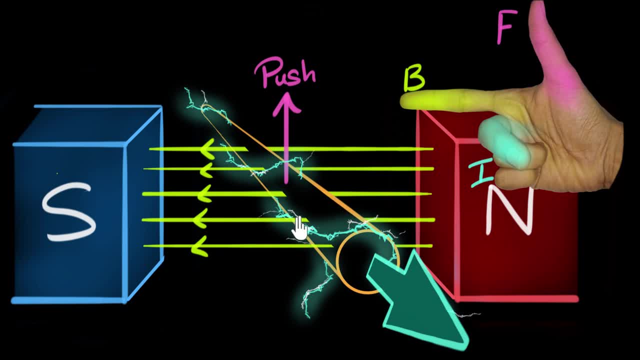 pushing the wire. so f for force. in what direction the wire is being pushed? the forefinger will tell us in what direction the magnetic field is, and the symbol for the letter for magnetic field is B. it's not M. I don't know why. then that's: the middle finger gives us the direction. 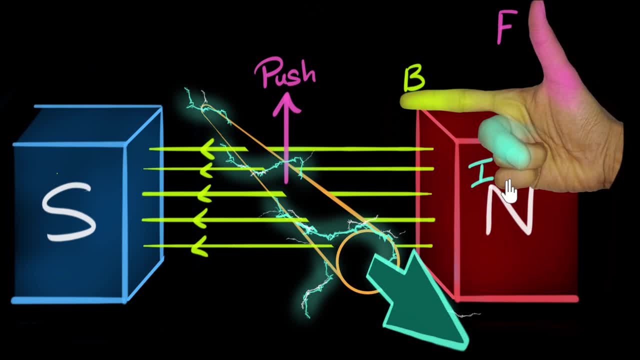 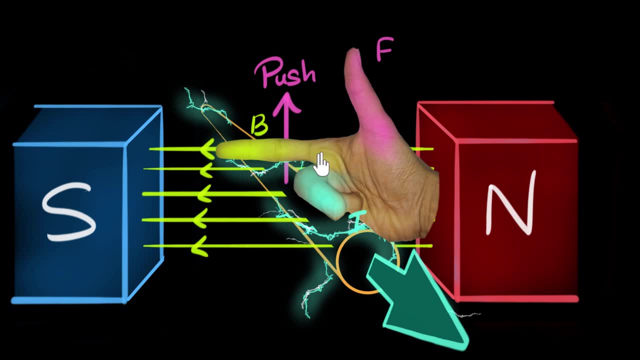 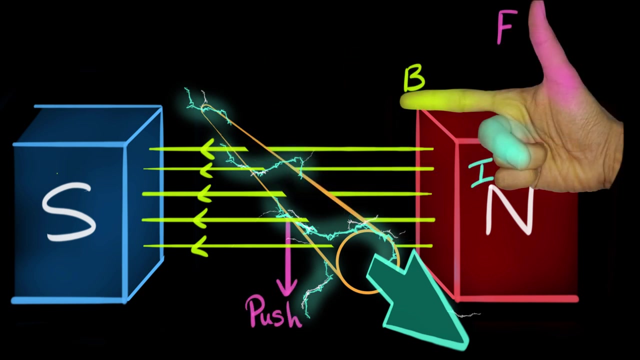 of the current. and so if you were to use this right hand rule over here, you can see the force is up the magnetic field, the forefinger is this way and the middle finger is pointing out of the screen, just as our current, and if you were to move this wire down, then this current direction would 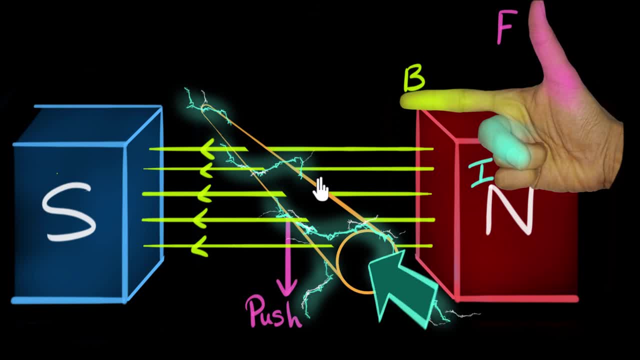 now reverse. now can you use your right hand generator rule one more time to convince yourself of this. make sure that the field forefinger is to the left, but this time make sure the thumb is pointing downwards and see what direction the middle finger points. go ahead, try this. all right if you have done it. 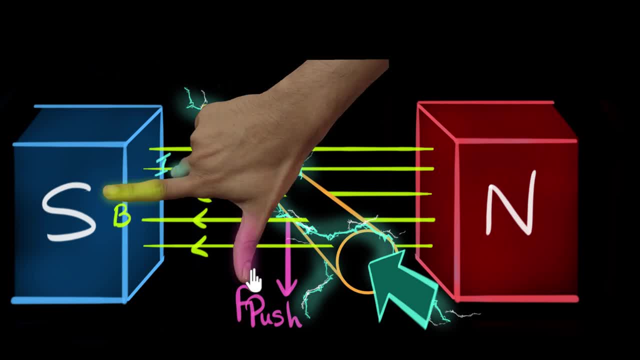 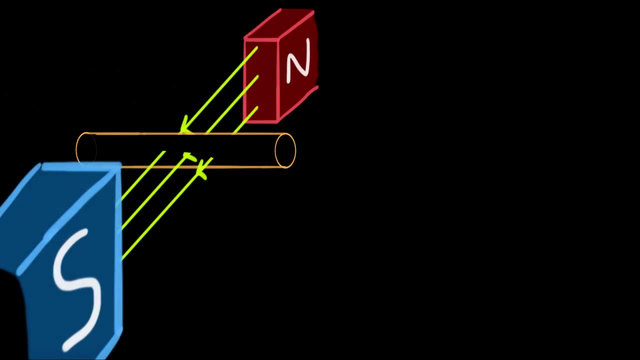 it might look somewhat like this: the force is down, magnetic field is to the left. now notice the current, that is, your middle finger is pointing Inwards into the screen, just like what we got here. so just for practice, let's take another example. here we have the magnetic field coming. 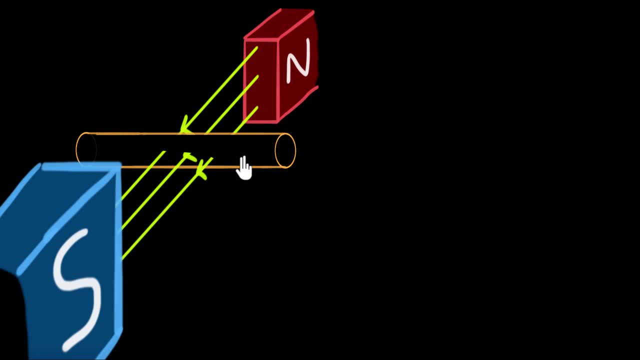 out of the screen this way and the conductor is going to be moved, let's say upwards. so we'll move the conductor up like this, cutting the magnetic field. can you figure out in what direction the current will run in this conductor? again, pause the video and see if you can try this yourself. 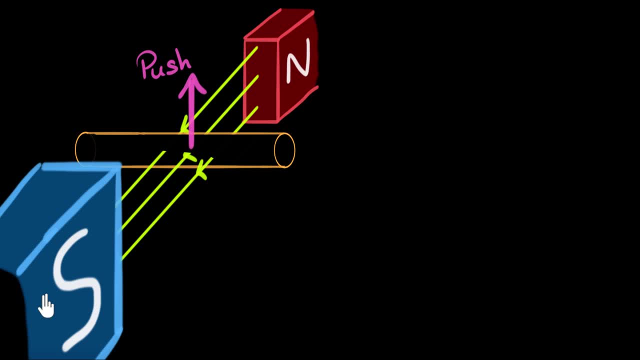 all right. we have to bring in our right hand, and if you align it according to the magnetic field and the push or the motion of the conductor, it would look somewhat like this: the forefinger points in the direction of the magnetic field and the thumb must point in the direction of the 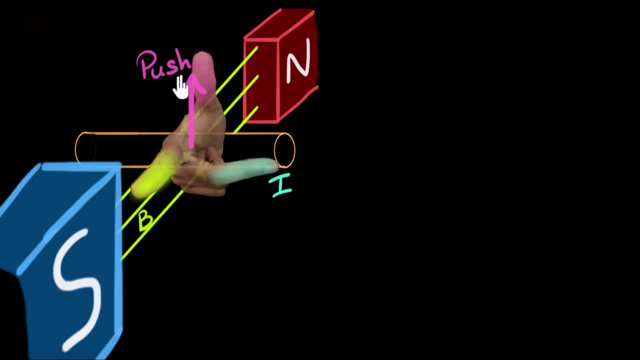 motion of the conductor in the direction in which we are pushing the conductor. then notice, the middle finger points to the right. that means the current in this conductor will flow to the right. so this is how we use our right hand generator rule to figure out the direction of the current when any conductor or any wire is moved in a magnetic field.